Of course, most of them will be encrypted, but if you are going to, for example, Starbucks or something else where they have free public wifi, you will be able to capture a lot of other people's traffic And, again, most of it will be encrypted, but there will most likely also be some unencrypted data. This, of course, is illegal just to capture people's packages and use it for maliciousness, But as a study case, it can be very educational to see traffic from a lot of computers in order to understand what kind of network packages is going back and forth through a network. 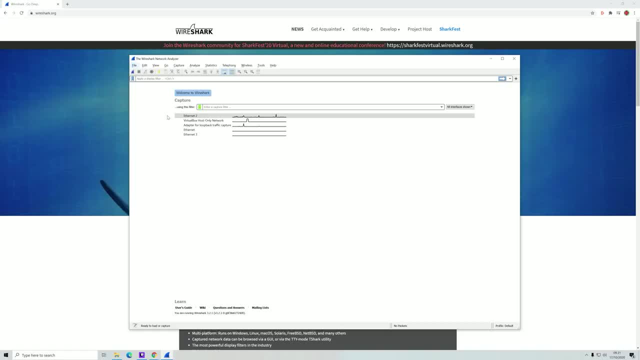 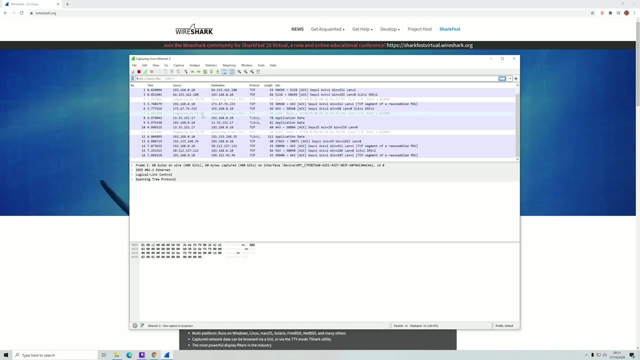 But for now we will just learn about the basics of the Wireshark. So we will be selecting the network that I have traffic on the Ethernet 2.. So click here And, as you see, it automatically got into capturing mode. So now it is capturing all the network traffic that is going through and from my PC. 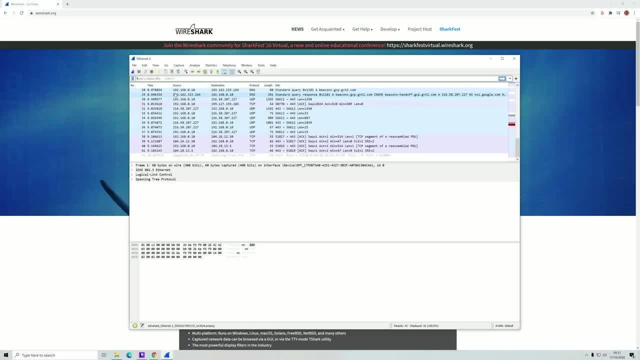 And if I just click here, it will stop, and then this will be our amount of packages that we just captured, And if I want to capture more packages, I can just click here again and start a new capturing process. But for now let's look at these packages. 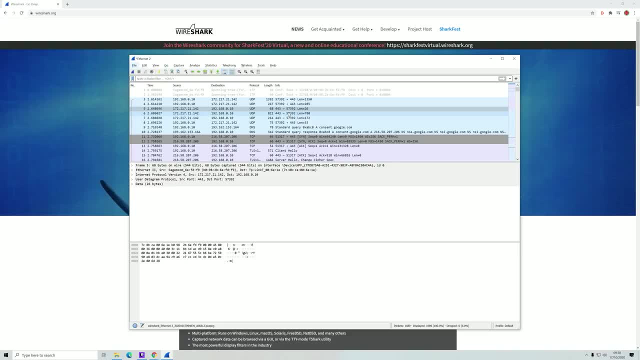 So now that we have captured some network traffic, we can see an overview right here So we are able to see the time of when these were captured. We can see the number of the packages, We can see the source. So what device, IP were they coming from? 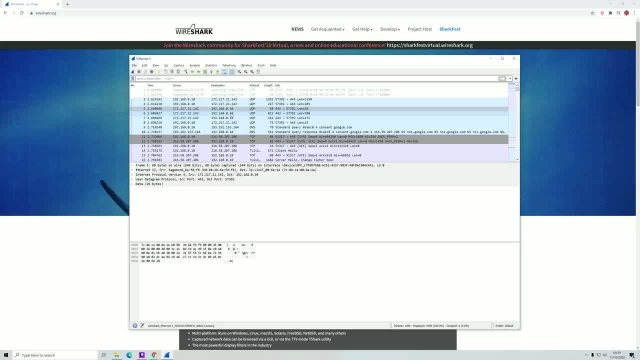 The destination, what IP is they trying to reach, Their protocol, Some length of the package and additional info. So if you are unfamiliar with networking in general, such as IPs, different protocols, I recommend that you watch my network basics series, which I will have a link to in the top right corner. 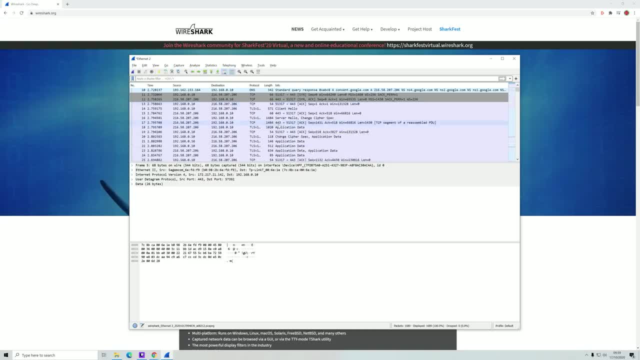 But for now let's try to look at some filters. So, as you see here, there is a lot of packages being captured Just during the time that we had it running, which were a very short amount of time. So you will see that you are capturing a lot of network traffic because all your applications on the computer is running in the background sending information back and forth. 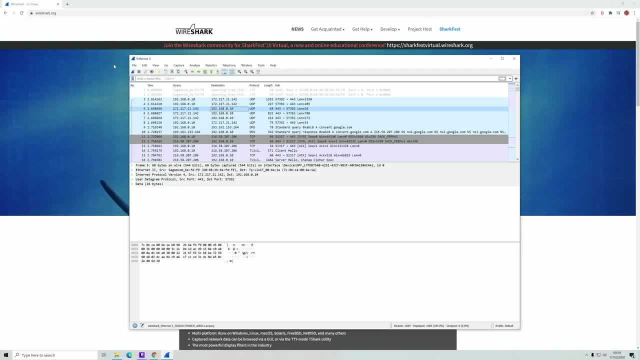 So just because you are not doing anything in your browser, your computer is still communicating a lot with the wider internet or your router. So, and especially if you are scanning a wireless network Where you have your network card set to monitor mode, You will of course see all the traffic from all devices on that network. 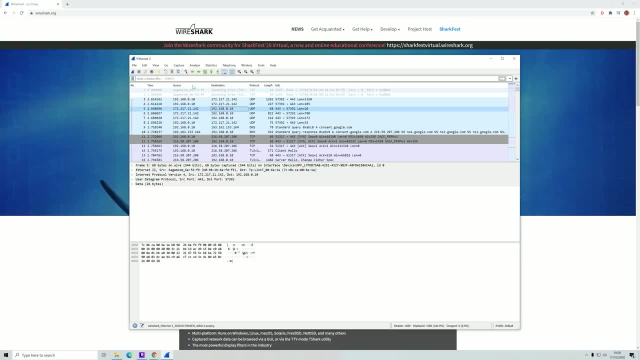 Which will add up a lot. But you can do filtering on packages in Wireshark. So, for example, if you are only interested in packages using the TCP protocol, You can just write TCP here And then you will only see TCP protocols. You can do the same for, for example, UDP. 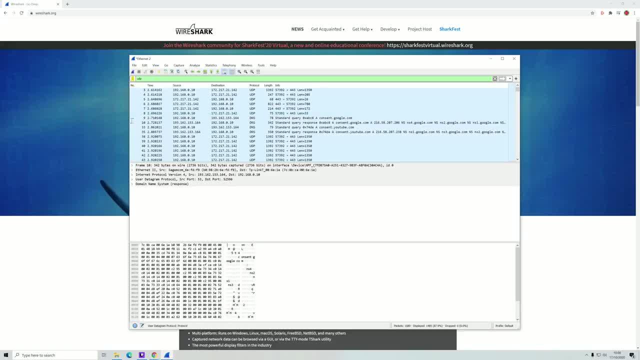 And you will only see these types of protocols If you are interested in packages, for example, going to a certain website And you know that it will contain a certain word, You can. let's see if we start capturing here. I will try to navigate to YouTube. 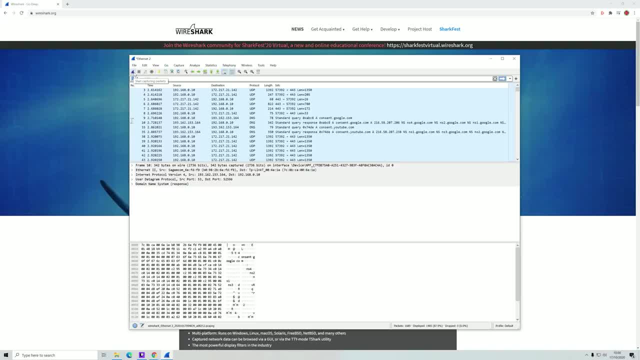 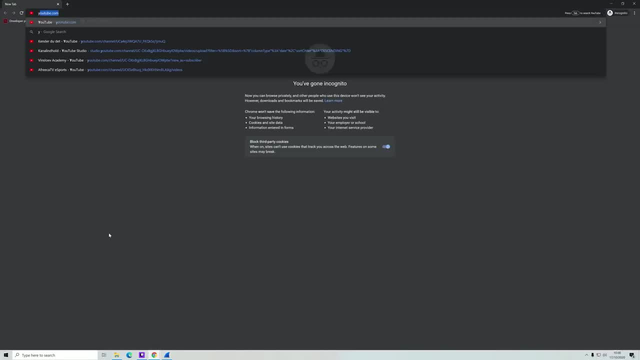 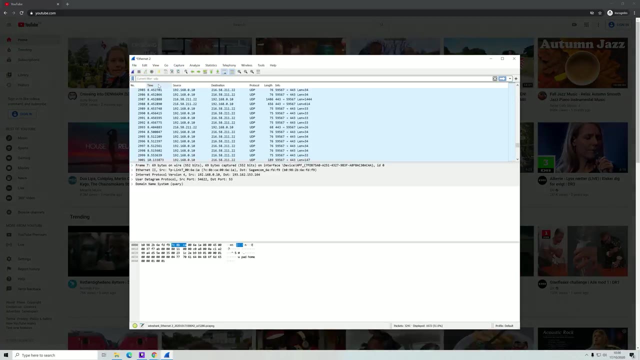 And find the package afterwards with the word YouTube containing. So we will start capture here, Continue without saving. Then I will go into my browser Into a new window Type YouTube, And if I then go back here And stop this capturing, 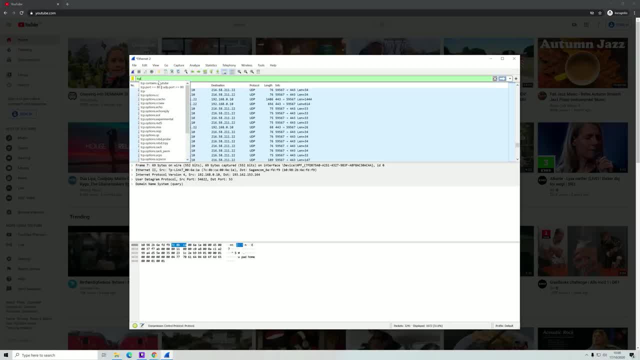 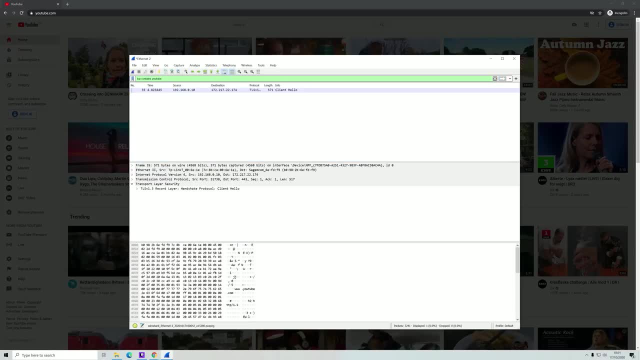 I can go up here and type: TCP contains YouTube. Then I am filtering now on packages with the TCP protocol That contains the word YouTube, And here we found one package That is going to one of YouTube's servers, And this is using the TLS 1.3.. 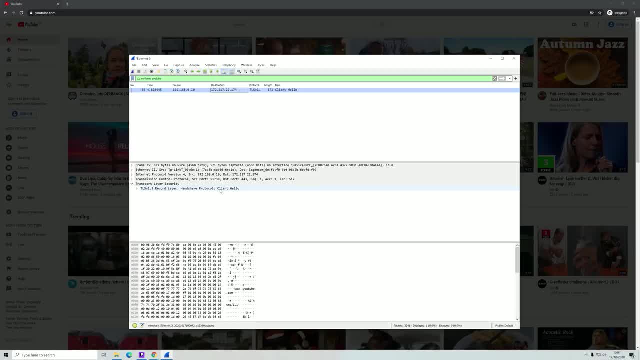 This you can also learn more about in my network series, Where we are basically just saying hello as a client. And the reason why this package showed up Is because, if we look at this additional info here, We see that the URL YouTube is present. 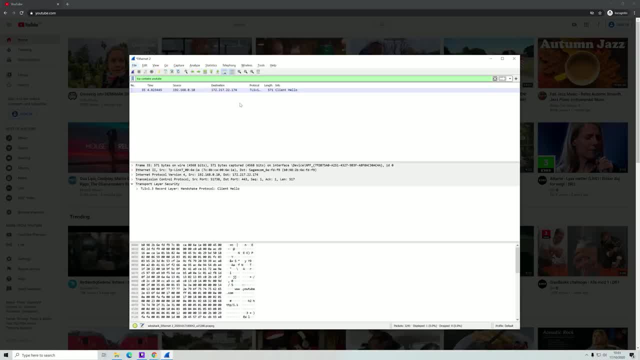 So let's say that I want to find all the packages That my device sent to this particular IP, So I will see if there are more packages That are not containing the word YouTube, Which were the filters that we used on this IP. 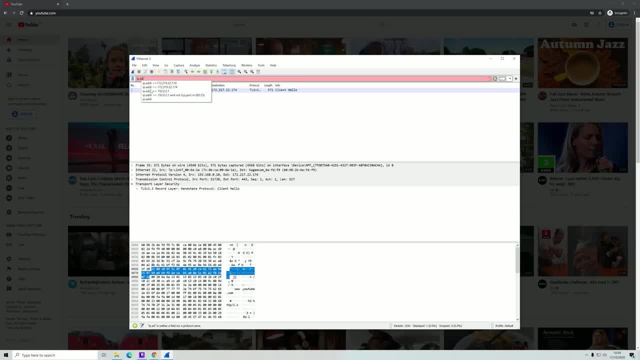 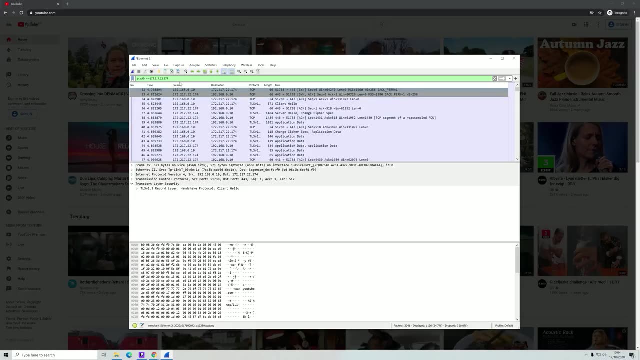 So instead I can type IPaddress- Let's see Address here And let's see It's 17.. So by typing IPaddress, Double equals and the IP here, Let's try to hit enter And, as you see, There is a lot of packages. 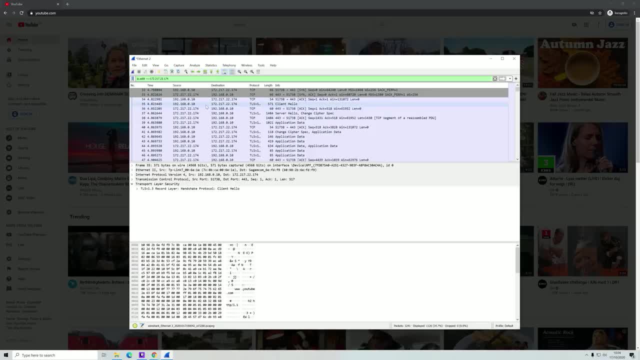 Going back and forth My device and the YouTube server. So here we see the package Where the IP is as destination. But it is also sending packages back to my computer, Because when I am hitting a URL, I am just saying to a server. 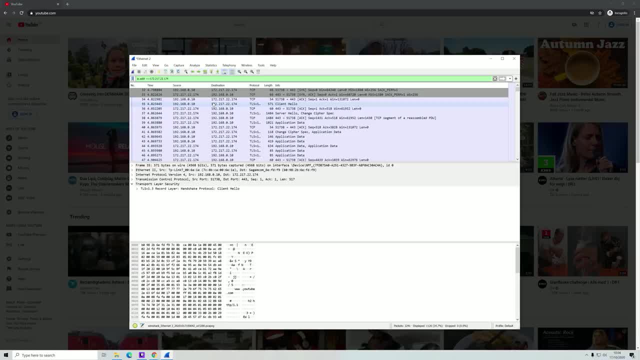 I need the information that you have here, And then it is sending it back to my IP. That is why we see that here It is the source, The server, And my computer IP is the destination of the package. So here we can see a lot. 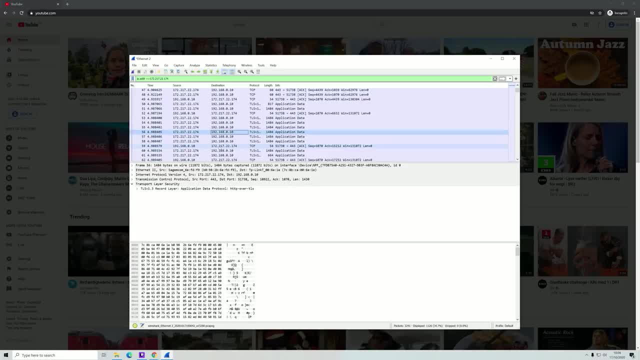 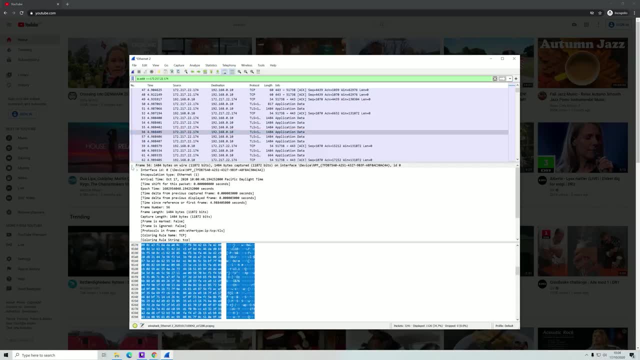 But let's try to go into one of these Right here And, as you see, There is a lot of garbage data in this, But you can also, For example here, Transmission. Here you can see The port that were used. 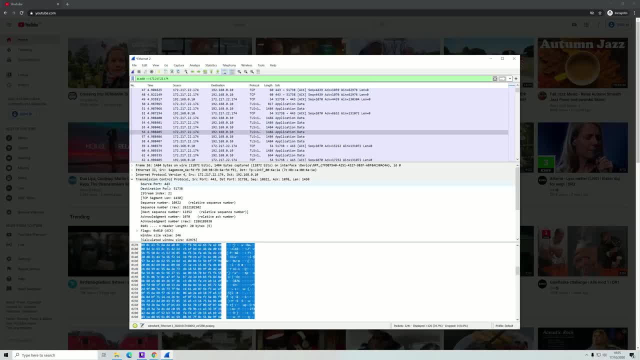 Normally all web traffic is going on the port 443.. And you can see Some of the size of the packages And also, if you are interested in the time stamp, How long it took To make the communication. So now let's try to see if we can find some traffic. 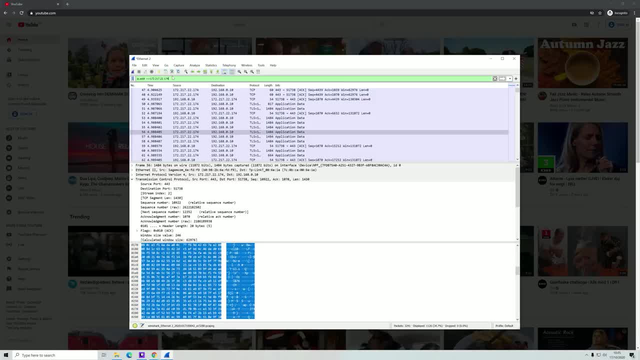 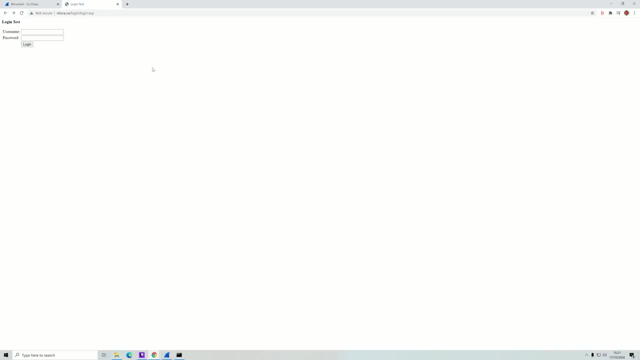 That is unencrypted, Meaning that We are able to read the data being sent, Because it is not using standard encryption Over the internet. So to illustrate How we can capture unencrypted data, I have navigated to this On jQuery site here: 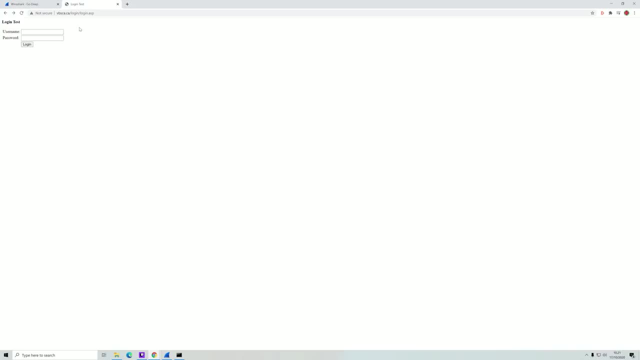 There is no encryption, No HTTPS on this. This means that the data that is being transferred From my browser to the server Is unencrypted And anyone listening in on these pages Can actually view the username and password. So let's try to test this. 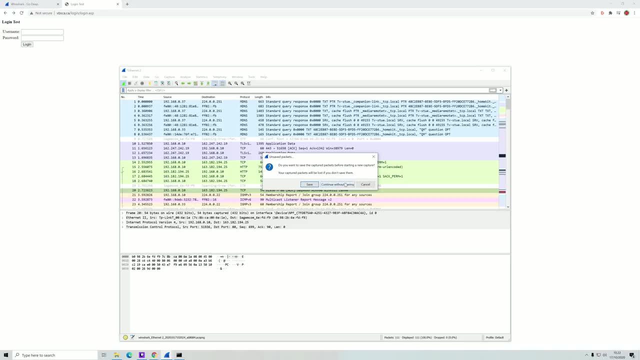 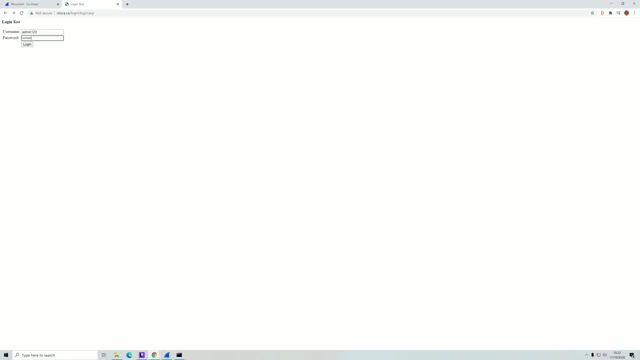 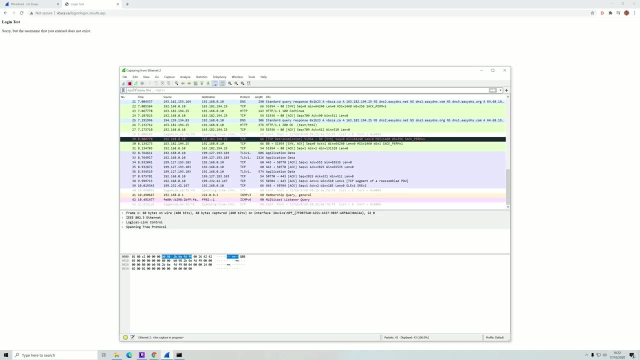 So we head up to Wireshark, We make a new capture, Then I enter the admin 123.. Admin 123. And click enter, And then it will see that Our user doesn't exist. But for this case It is no problem. 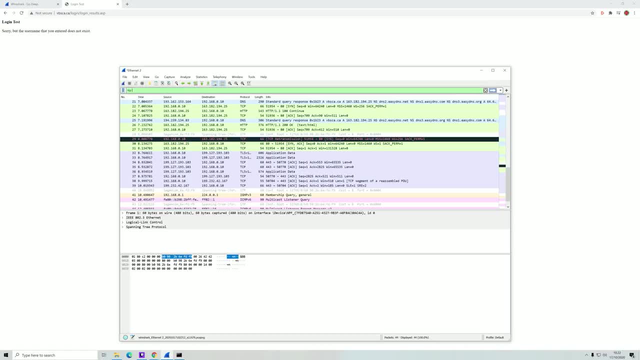 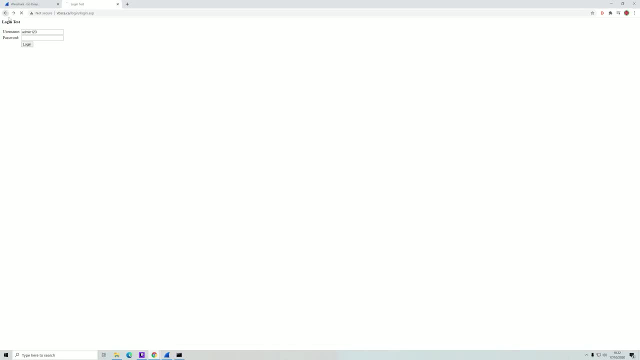 So, now that we have entered this, We will try to search for CCP That contains The username that we entered. I think that we can actually. Let's just try to search for username Instead of the actual username, Just to illustrate that. 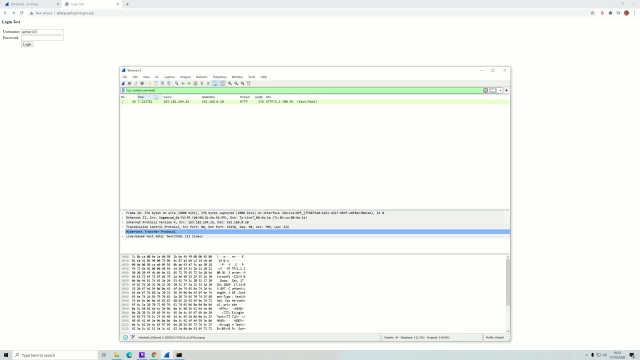 People that is listening in Can just find that data. So we find one package And let's see here Username server Microsoft. Sorry, but that username were not, So let's see what it does If we do like. so Let's see what it came under. 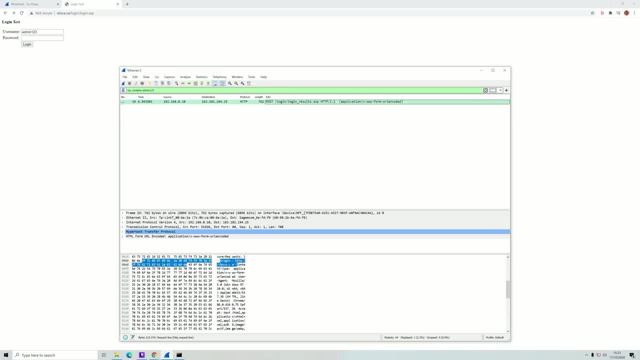 So here we have the post request And since this is unencrypted, We can see here, So it actually send it under Text username With a space, And that is why our search didn't find it, And the password is admin and 123. 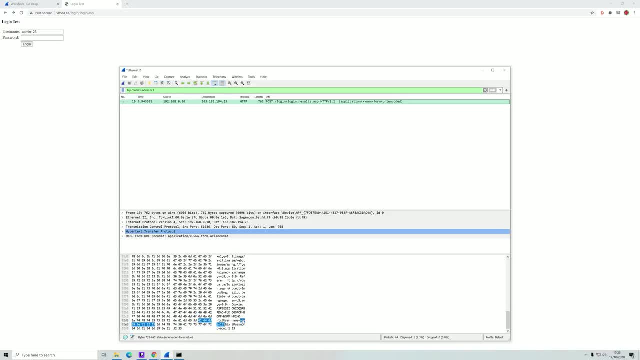 So here we can see that If anyone were listening in on this, For example, if I was on a wireless device And I tried to log in On an unencrypted site, They were actually able to see my information, And this is the same for credit card information. 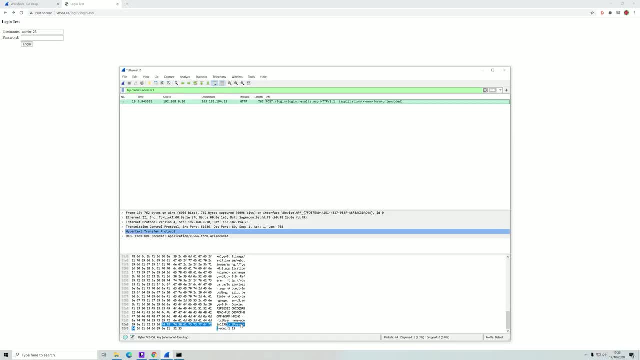 And all kind of information That you put on a site That is unencrypted. So be aware of this when you are using And browsing online. So, as you have seen Through these small examples, This is only the very basics. With Wireshark, it is capable of a lot more. 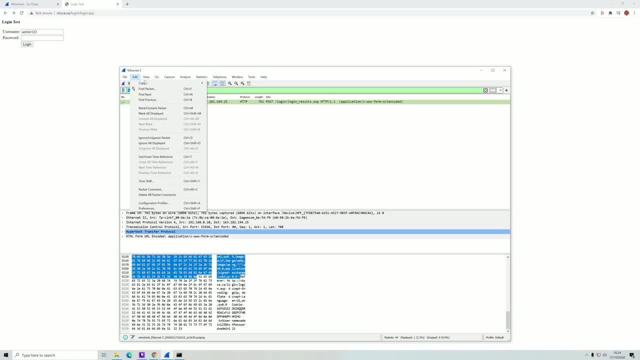 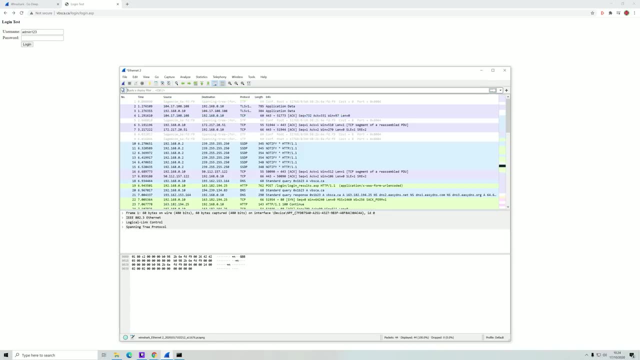 You are capable of making statistics And all kind of advanced packages And filtering, But I recommend that If you are interested in Wireshark in general, That you navigate to the site And see the user guide to learn more about The more advanced stuff that you can do. 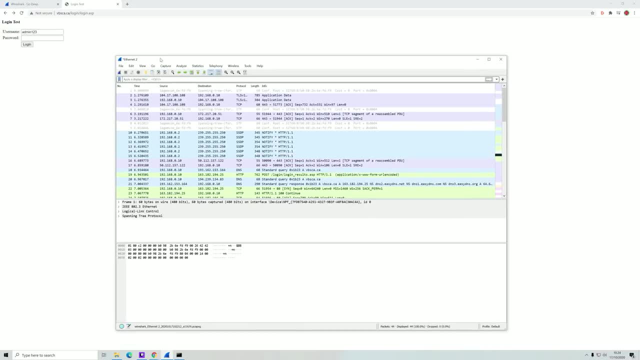 But now you have Been introduced To the basics That enable you to do some network analysis, Either on your own machine Or on your own local network, Just to get an idea of What kind of packages Is actually being transferred from and to your device.